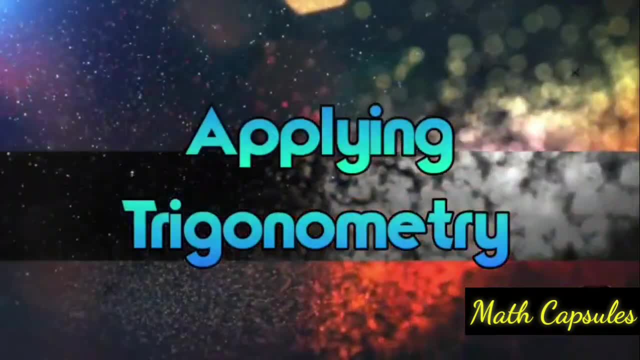 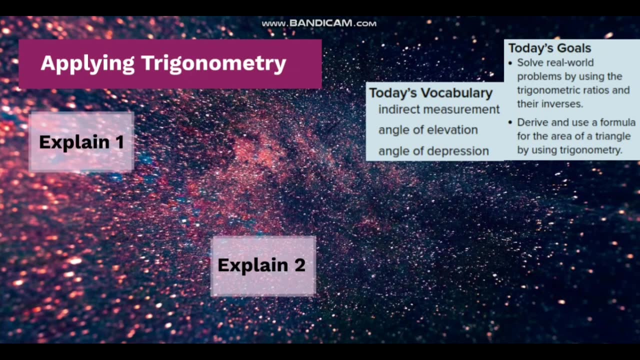 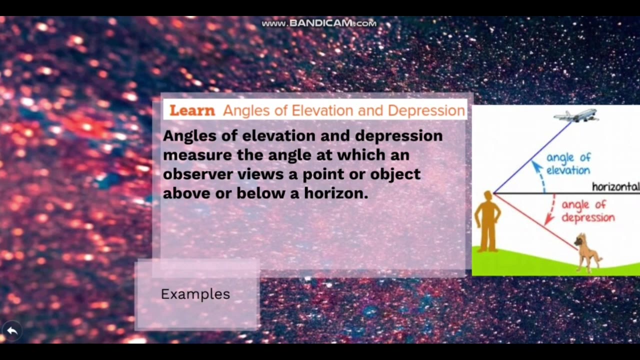 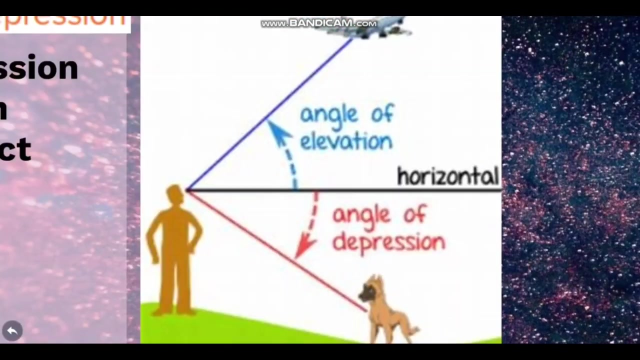 In this video we are going to solve real-world problems by using the trigonometric ratios and their inverses. The first thing to learn is angles of elevation and angles of depression. that measures the angle at which an observer views a point or object above or below the horizon. So if you are looking at a 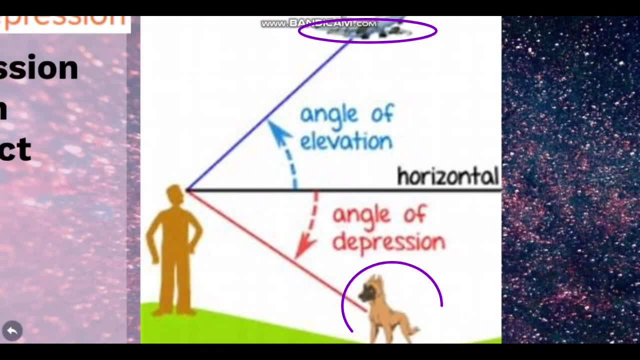 plane up there and a dog below the sight here will make an angle of elevation with the horizontal line in front of the eye with the other side, which is the sight of the plane. These two sides make an angle of elevation. The other side, where you're looking at the dog, makes an angle of depression, with 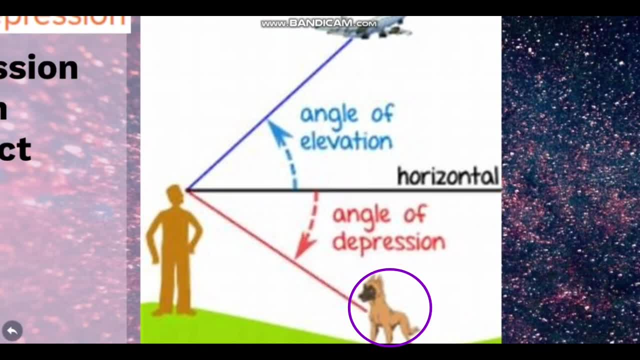 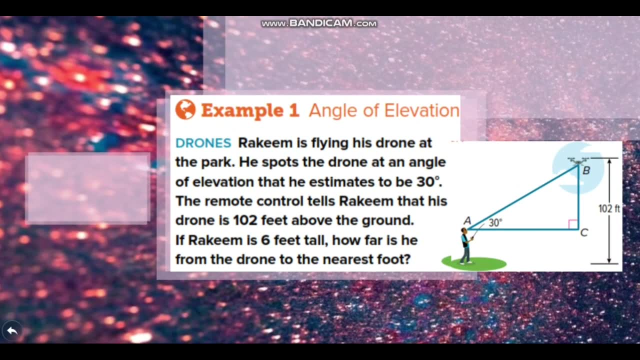 the horizontal line in front of your eye. Now let's look at this example. Rakeem is flying his drone at the park. He spots the drone at an angle of elevation that he estimates to be 30 degrees. The remote control tells Rakeem that his drone is 102 feet above the ground. If Rakeem is 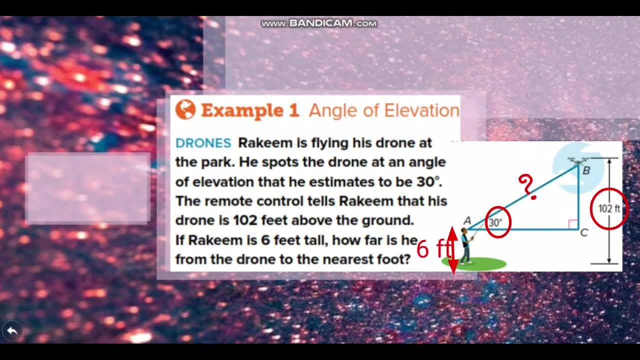 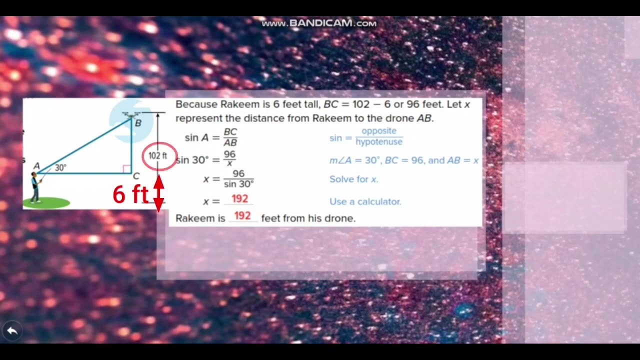 6 feet tall. how far is he from the drone to the nearest foot? This means that we need to find the hypotenuse length of this triangle, because Rakeem is 6 feet tall, this means that Absc is 102 minus 6, that is 96 feet. Now let X represent. 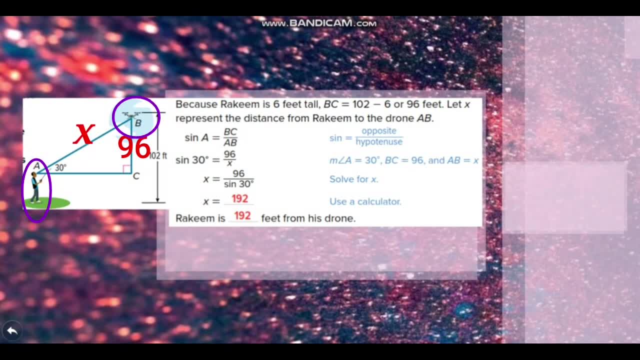 the distance from Rakeem to the drone AB, which is the hypotenuse length. So what relation relates the angle 30 with 96 and the hypotenuse x? 96 feet is the side of 30 degrees and X is the hypotenuse, so the relation is the sine. 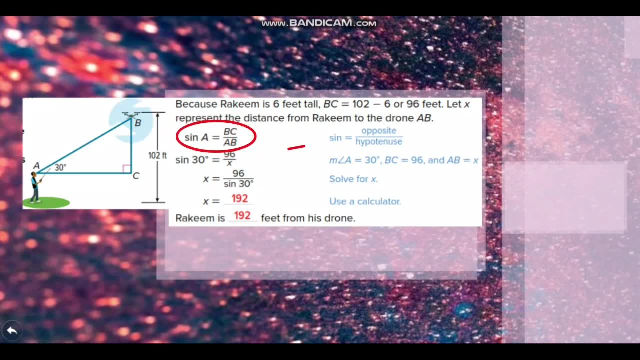 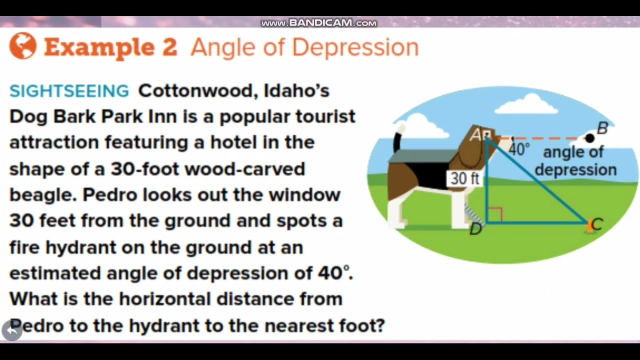 function because sine 30 equals 96 over X, so we can find the X by solving for X. you will divide 96 over sine 30. the answer will be 190, two feet from his drop. another example: cottonwood in a house dog bark Park Inn is a popular